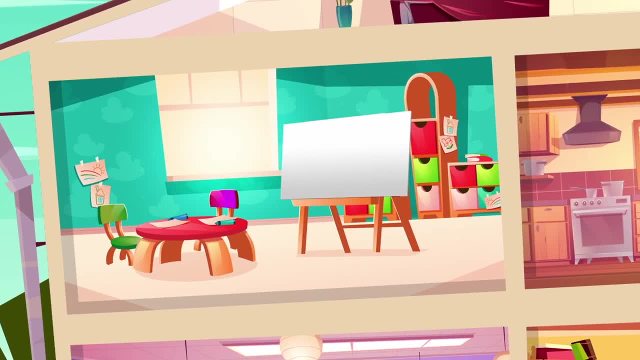 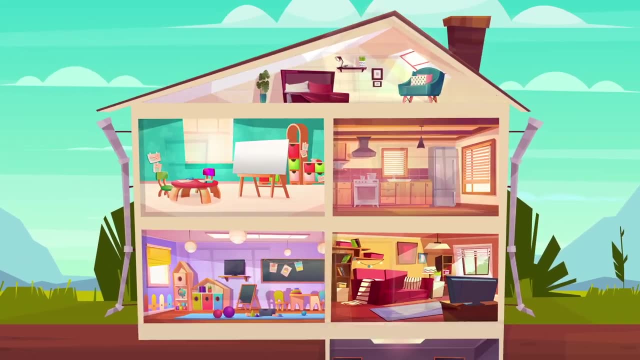 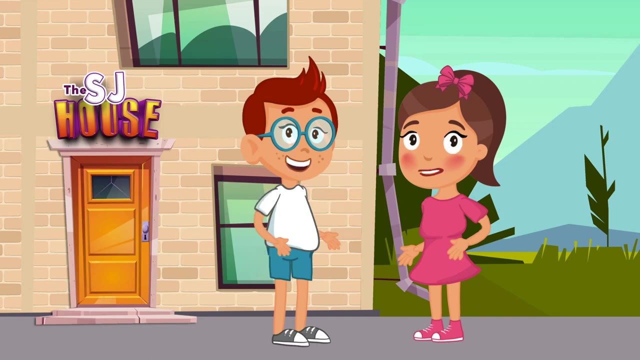 Hello kids and welcome to our show. Hey kids, hello, How are you today? We hope that you are doing fine. Thank you for all your wonderful messages and paintings that you send us. Yeah, we just love hearing from you. Do you remember the other day that we went to the planetarium and we promised you that we will do an episode with simple things we can do to protect our planet? 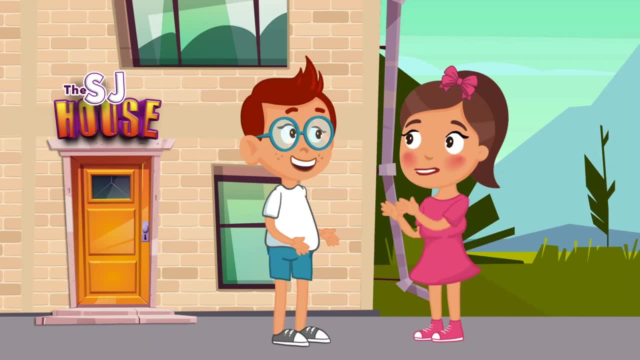 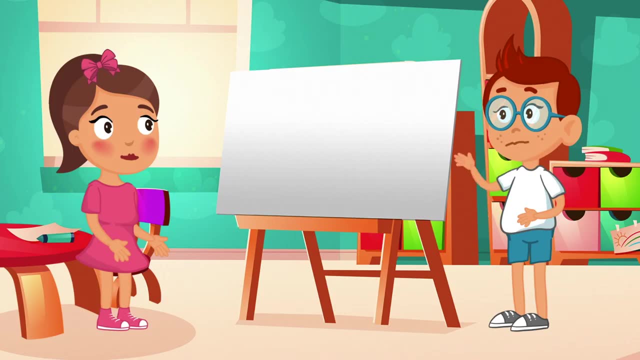 So that is it. Today's episode is just about that. Shall we go inside? So here are some very simple things we can do every day and will affect positively. Let's start. First of all, we can turn off the tap while brushing our teeth or while taking a bath. 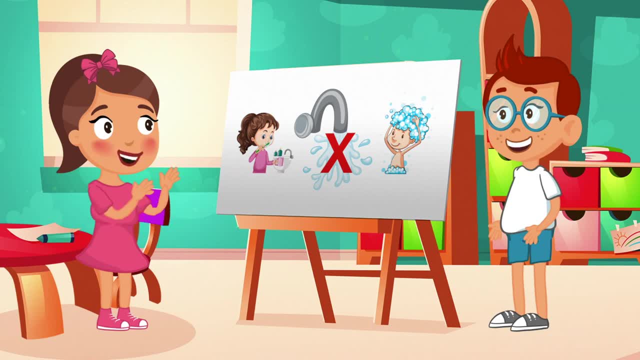 It does not sound so important, but by doing this simple move, we can save millions of gallons of water per year. Isn't that amazing? That's right, Sasha. The water is so important for our life. Next thing we can do is to reuse, transform things instead of throwing them in the trash cans. 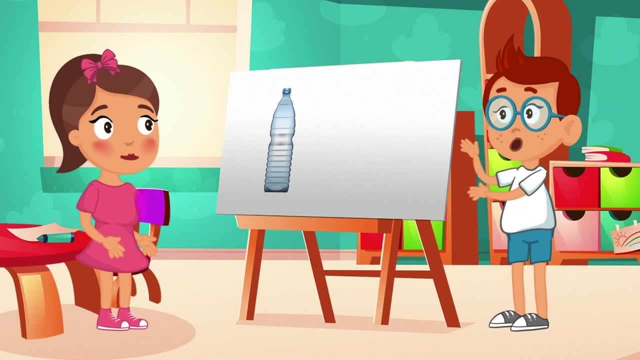 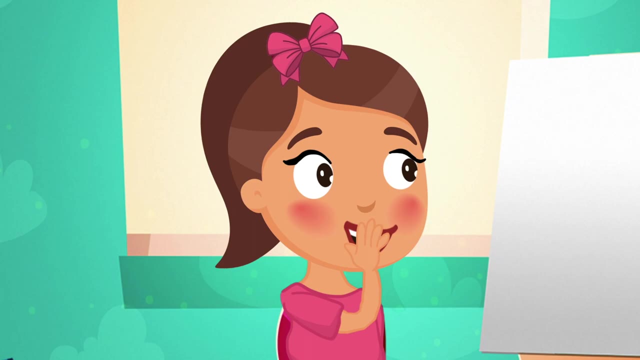 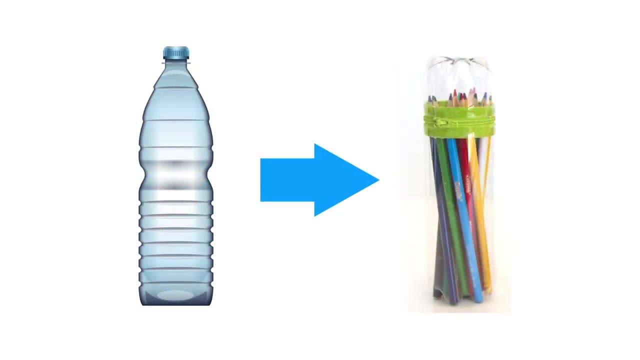 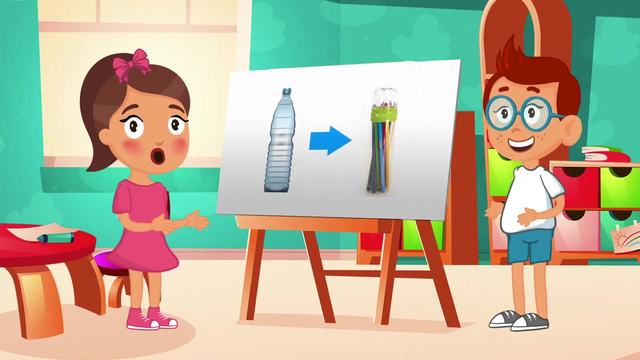 For example, instead of throwing away a plastic bottle, we can keep it, and by using our imagination, we create many beautiful things for us and our friends, Like this very beautiful pencil holder. Wow, Jason, This is so cool. Hey, kids, before throwing away something that seems useless, you can get ideas from the internet of how to transform it back to something very beautiful and helpful. 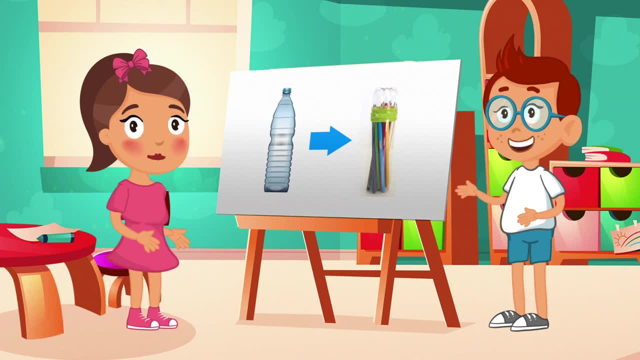 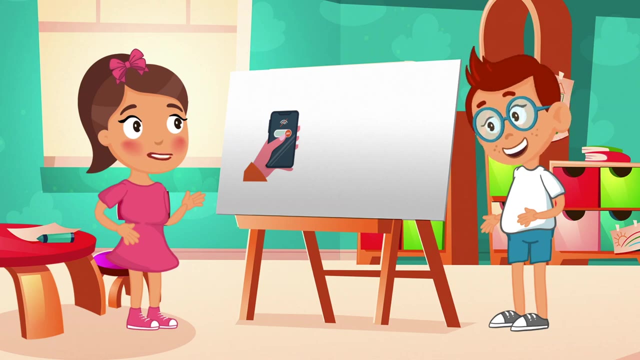 By doing this, not only are we being creative, but also we save the planet from extra garbage. Next simple thing we can do to protect our planet is to turn off all electric devices, instead of just put them to sleep mode when we don't use them. 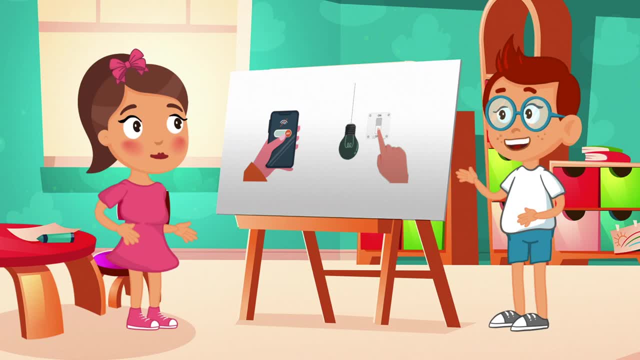 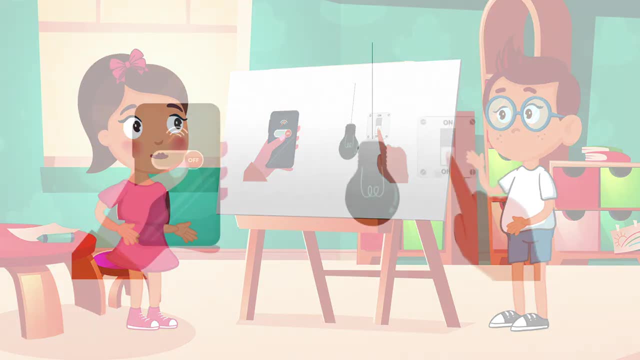 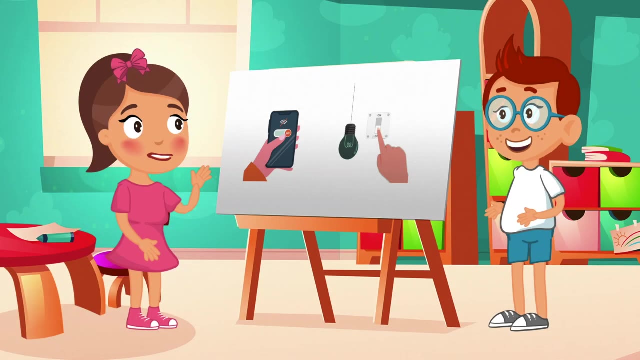 Also turn off the lights when we leave a room. This simple move will save electric energy and protects the planet from pollution, because in order to produce electric power, we drastically affect badly the environment. That's right, so keep in mind to turn off the light and shut down your computer when you leave the room. 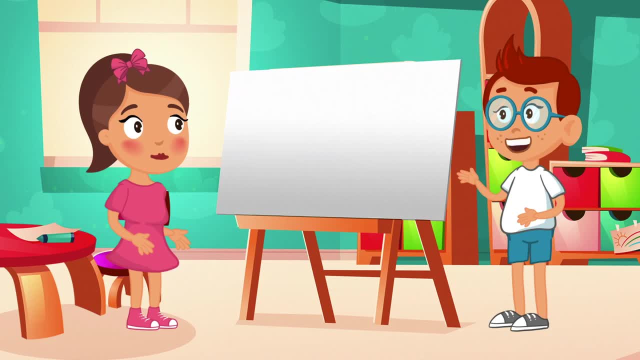 Finally, the most important but very simple thing to do in a daily basis that will protect our planet is, of course, to recycle Instead of throwing away everything in a trash. can we can separate these four different materials from our garbage? Can you please tell us, Sasha, what are these four materials? 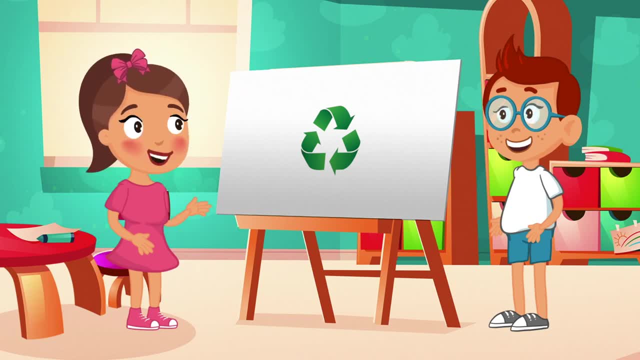 Sure, Jason. thank you. These materials are: one paper, like boxes, old magazines, etc. Two plastic, like the water bottles. Three, glass, like wine bottles or bottles from perfumes, And four aluminum, like most of the soft drink cans. 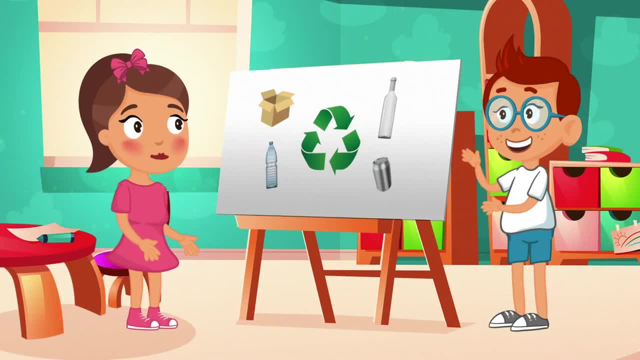 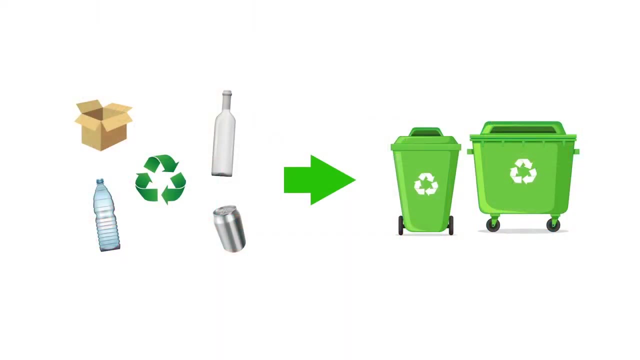 All we have to do is to separate them in a different bag or container and throw them away in the special trash cans that have the recycle symbol on them. And, of course, you can always ask for help from your parents If you don't know what to do with a specific material. you can also invite your parents to recycle too. 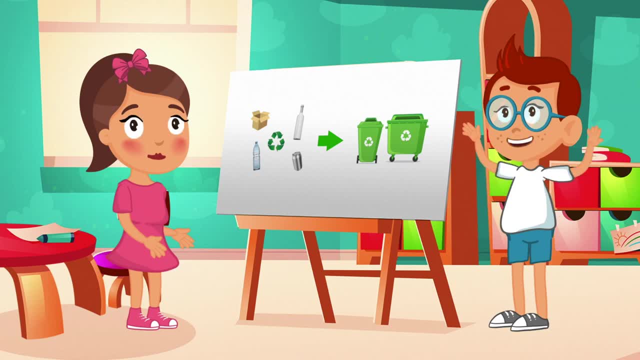 So you can do this as a family and feel proud that you support saving the planet. Hey kids, what do you think Isn't that easy? Let us know in the comments below what, of all these four simple things, you've managed to do. 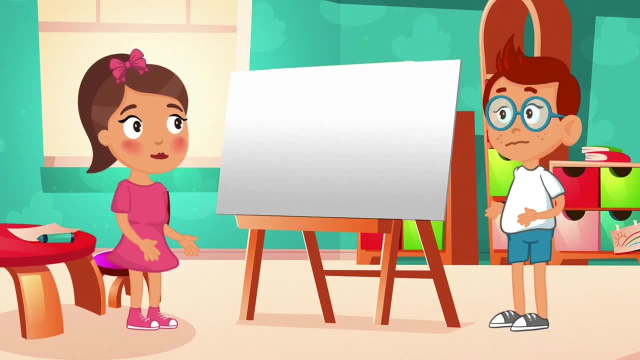 Yeah, and now Sasha, it is time to say goodbye to the kids. Hey, here's John and Calvin. Bye kids. Yvonne Devonnie, I see you, Hello there. Here's Nicholas and Becky too. Hello kids.